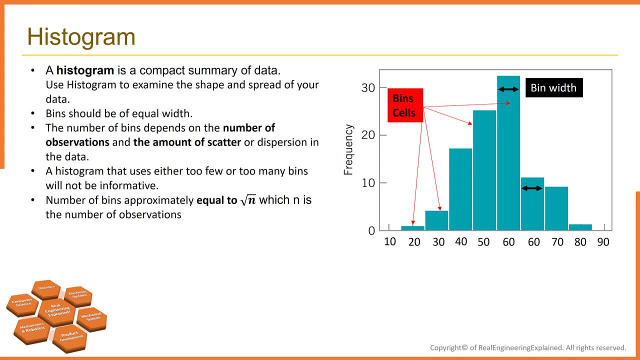 display can be developed. The number of bins depends on the number of observers in thatją observations and the amount of scatter or dispersion in the data. A histogram that uses either too few or too many beans will not be informative. Choosing the number of beans. 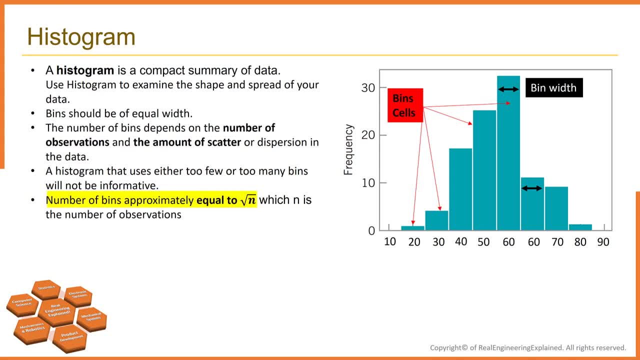 approximately equals to the square root of number of observations, usually works well in practice. Once the number of beans and the lower and upper boundary of each bean has been determined, the data are sorted into the beans and the number of observation in each bean is counted. 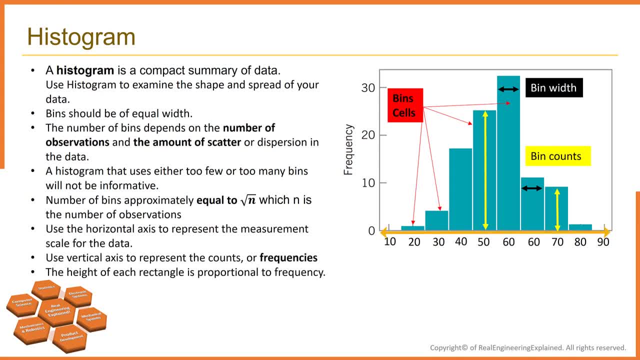 To construct the histogram, use the horizontal axis to represent the measurement scale for the data and the vertical scale to represent the counts or frequencies. For example, rectangles are drawn over each bean and the height of each rectangle is proportional to frequency. Okay, there is important note here. 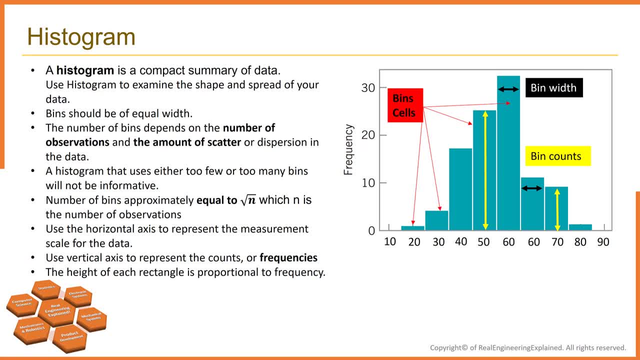 Histograms can be relatively sensitive to the choice of number and width of the beans. For small datasets, histograms may change dramatically in appearance if the number or width of the beans changes. For this reason, we prefer to think of the histogram as a technique best suited for larger datasets. 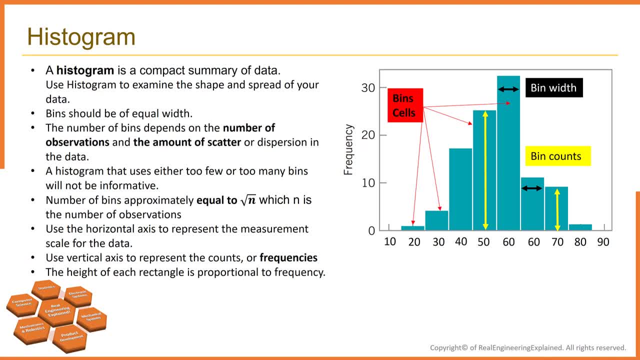 containing, let's say, 75,, 200, or more observations. So the histogram gives us some information about the shape of the distribution of data and also it gives us some information about the central tendency in the data and the scatter or variability in the data. 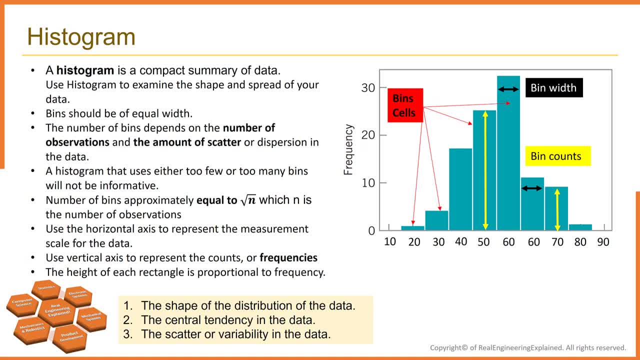 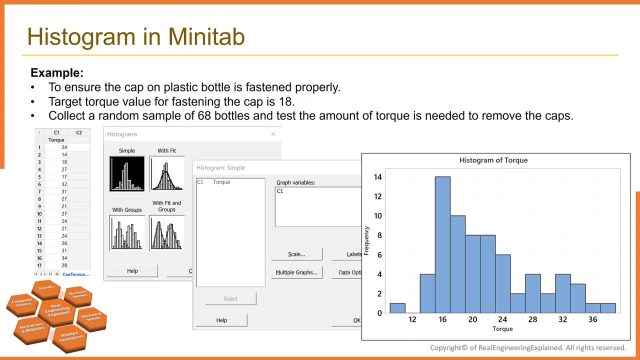 These are the main information that we can get from the histogram. Here is an example. A quality control engineer needs to ensure that the caps on the plastic bottles are fastened correctly. If the caps are fastened too loosely they may fall off during shipping. 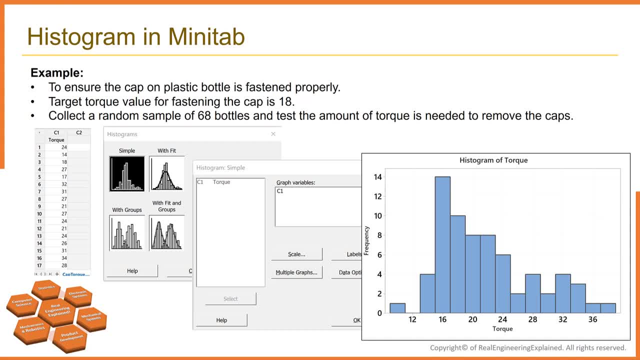 If they are fastened too tightly, they may be too difficult to remove. The target value for fastening the caps is 18.. The engineer collects a random sample of 68 bottles and tests the amount of the torque that is needed to remove the caps. 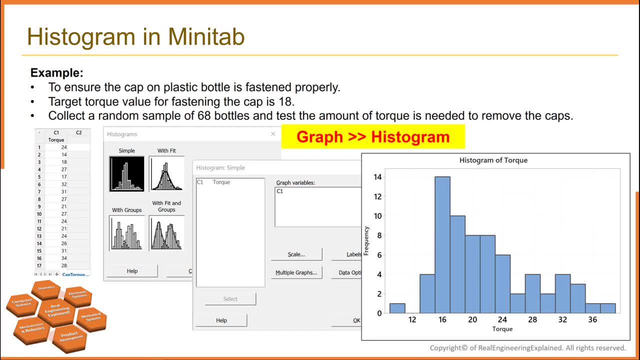 Here is the data To plot the histogram. go to the Graph menu and select Histogram, Then select Simple and then select Column C1 or Torque and finally hit OK. As part of initial investigation, we created a histogram of torque data to evaluate the distribution of data. 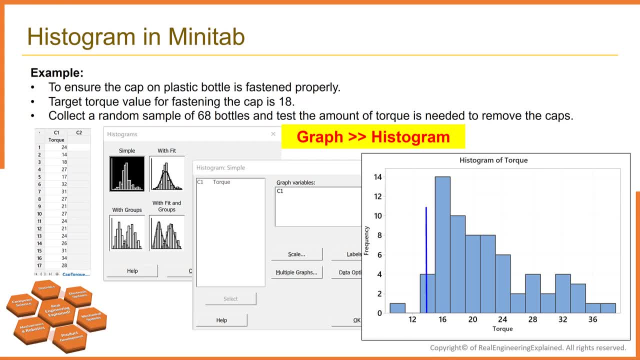 As we can see, most caps were fastened with a torque of 14 to 24.. Only one cap was very loose with a torque of less than 11.. However, the distribution is positively skewed is right skewed. Many caps required a torque of greater than 24.. 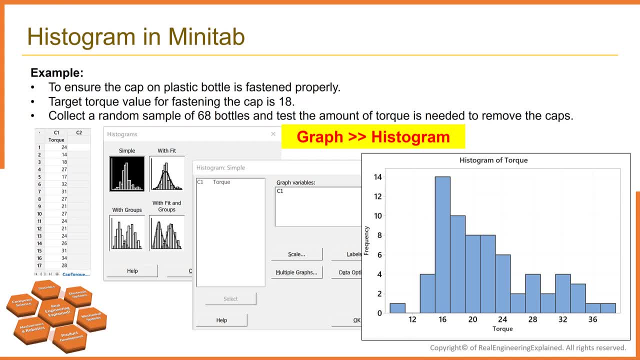 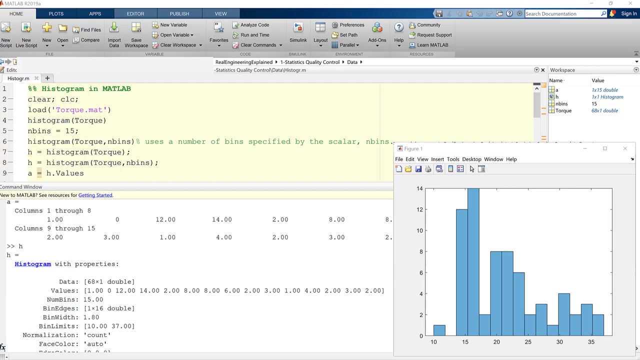 And 5 caps required a torque of greater than 33, nearly 2 times the target value, which was 18.. So you see that how histogram gives such useful information about shape tendency and variability of data. Let's plot the histogram of data in MATLAB. 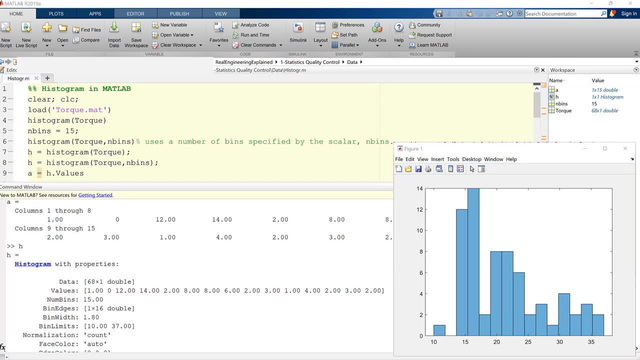 In MATLAB, the histogram function uses an automatic binning algorithm that returns bins with a uniform width to cover the whole range of observations. In MATLAB we use histogram function. In this function we can define the number of bins as well In this command. 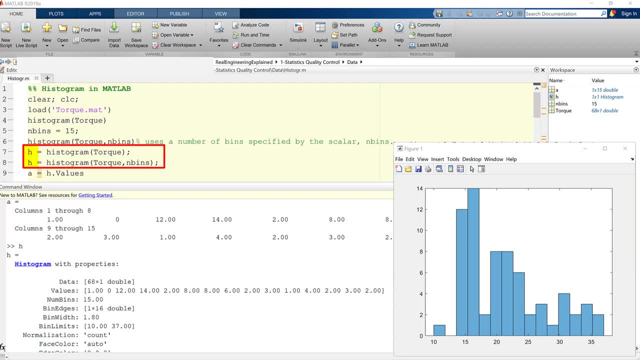 object H is holding histogram object and all its properties. If you type H you can get all properties. We can get the number of counts or frequencies in each bin by command Hvalues. This says the third bin includes 12 observations and the fourth bin includes 14 observations. 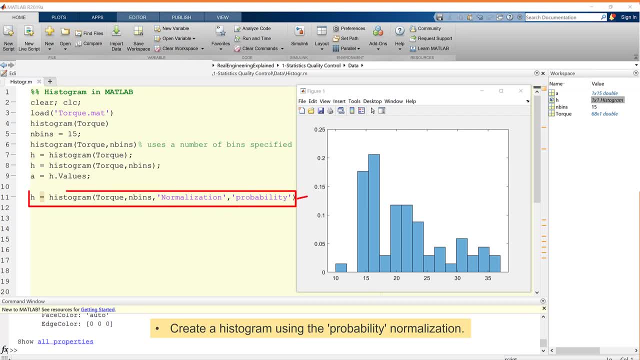 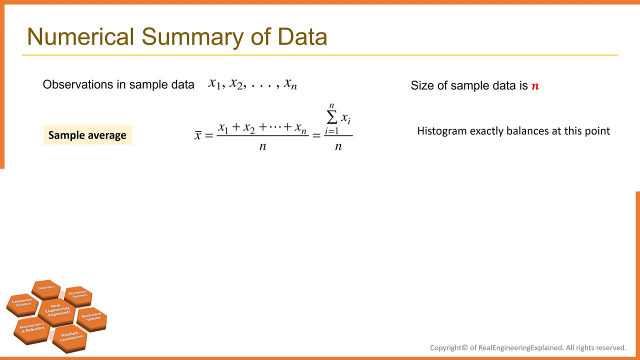 We can also create a histogram using the probability normalization, like this. The second topic which I would like to talk about is numerical summary of data. The histogram provides a visual display of three properties of sample data: The shape of the distribution. the shape of the distribution of data. 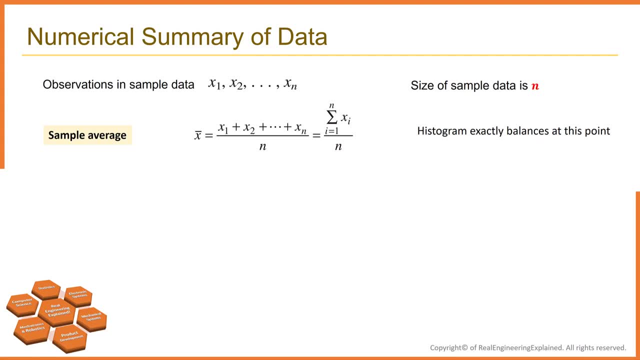 the central tendency in the data and the scatter or variability in the data. Assume x1, x2, until xn are the observations in a sample. The most important measure of central tendency in the sample is sample average. Note that the sample average 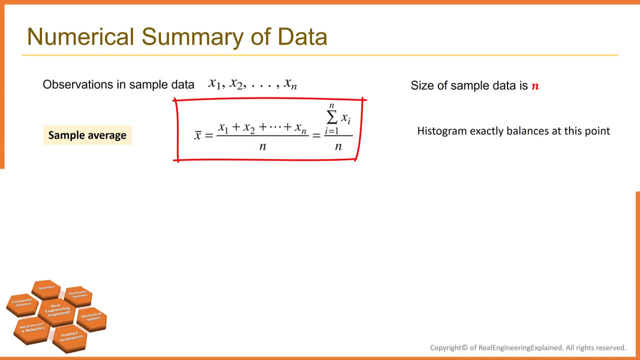 is simply the arithmetic mean in observations, summation of all numbers divided by the number of observations. The sample average for the data is the point at which the histogram exactly balances. So the sample average represents the center of mass of sample data. The variability in the sample data. 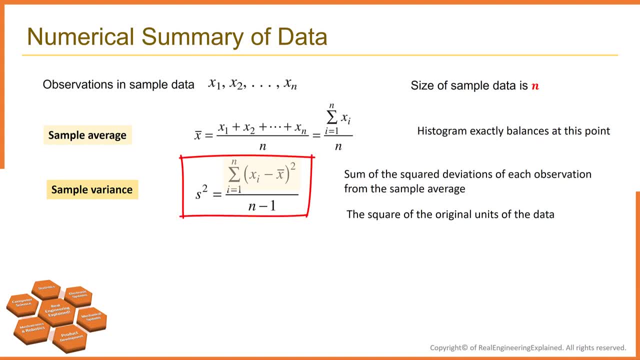 is measured by the sample variance. Note that the sample variance is simply the sum of the squared deviation of each observation from the sample average, divided by the sample size minus one. Generally, the larger is the sample variance, the greater is the variability in the sample data. 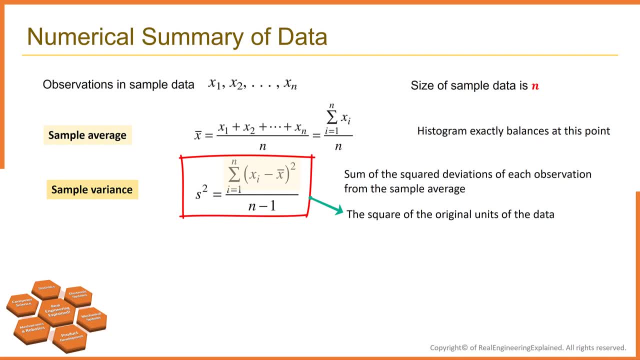 The unit of sample variance is squared is the square of original units of data. So, since it is often inconvenient and awkward to interpret, we usually prefer to use the square root of s squared, which is called sample standard deviation s, as a measure of variability. 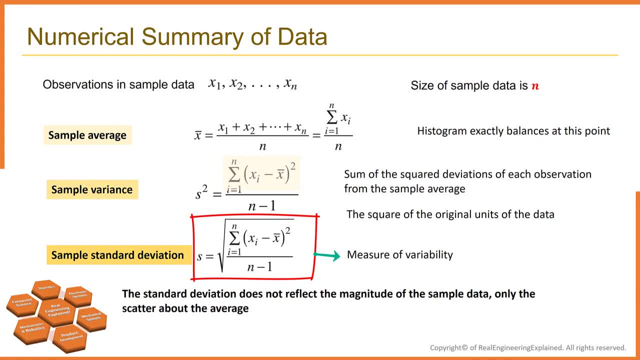 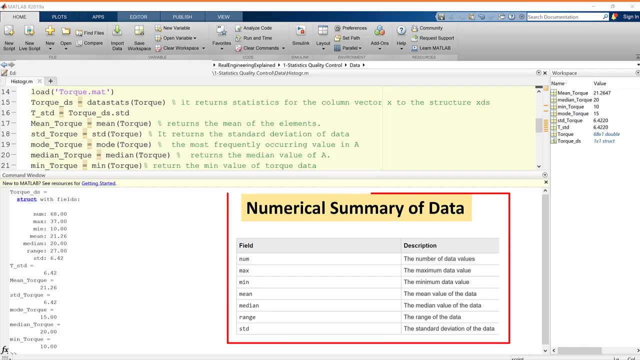 Please note that the standard deviation doesn't reflect the magnitude of sample data. It only gives information about the scatter of data, about the average. That's it. Let's switch to MATLAB to see how easily we can get these numerical summaries from the Torque data. 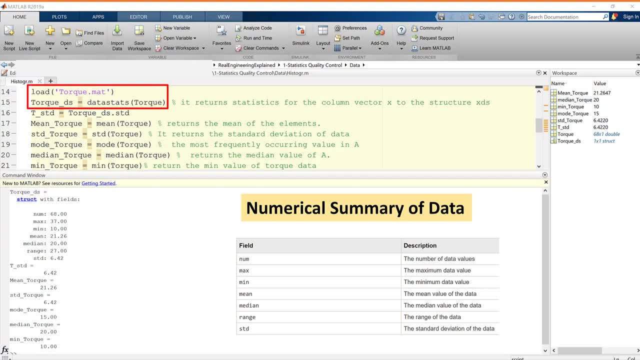 Here we load the Torque data. With data stats function we can get the numerical summary of data and then save in Torque underline s. Then with this line of code we can access to the standard deviation of data. This line returns the mean of data. 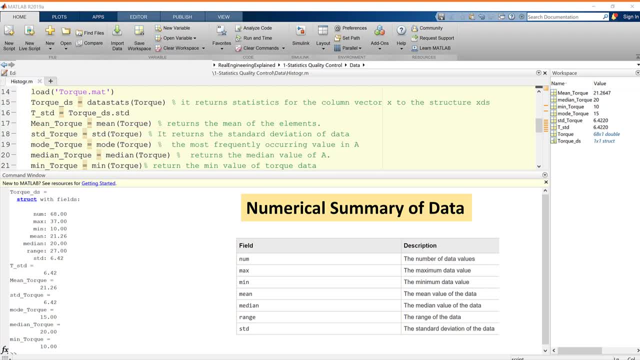 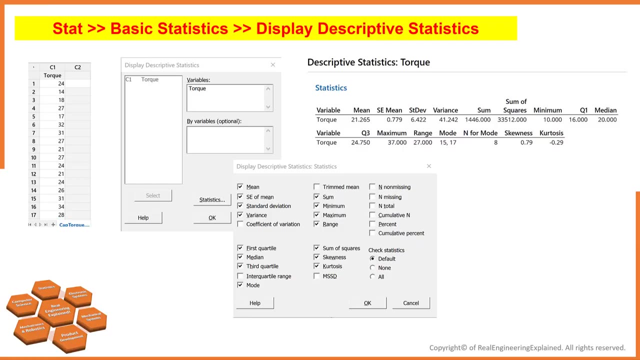 And this line returns the standard deviation of data. We can also get mode, median, mean or max of the data. Please note that the median is the median number in a sorted ascending or descending list of numbers. You can get the similar result from the Minitab. 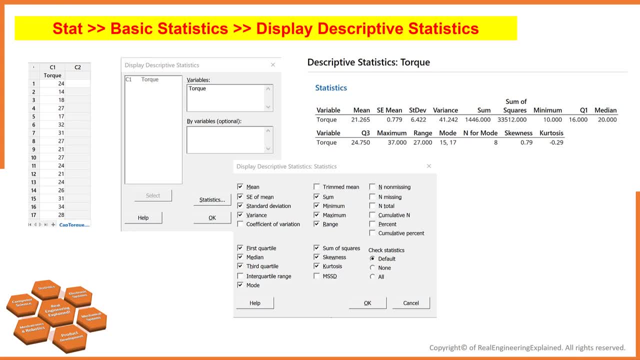 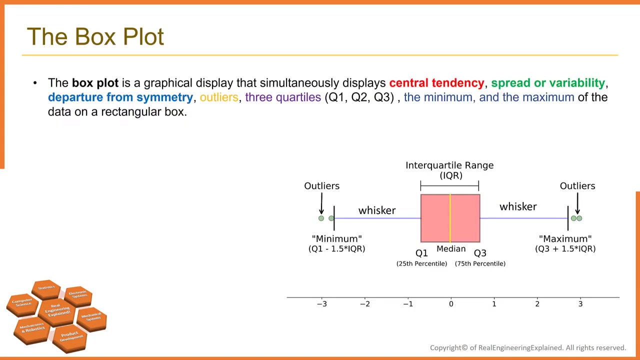 Go to stat and then basic statistics and then display descriptive statistics. In the variables section select Torque or column C1., Click on statistics and select those information that you need And then finally hit OK. Here is the summary of data. The third topic which I would like to talk about. 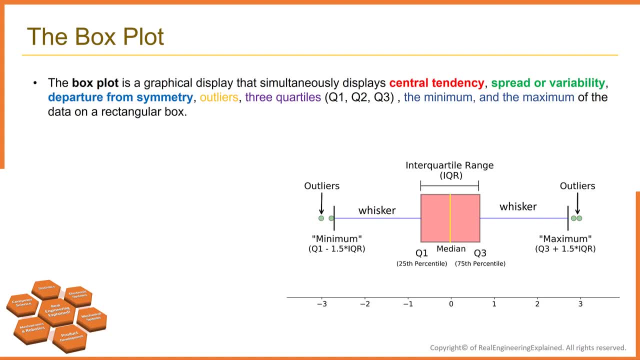 is the box plots. The box plot is a graphical display that simultaneously displays several important features of data, such as location or central, tendency of data, spread or variability, departure from symmetry, identification of observations that lie far from the majority of data. These observations are often called outliers. 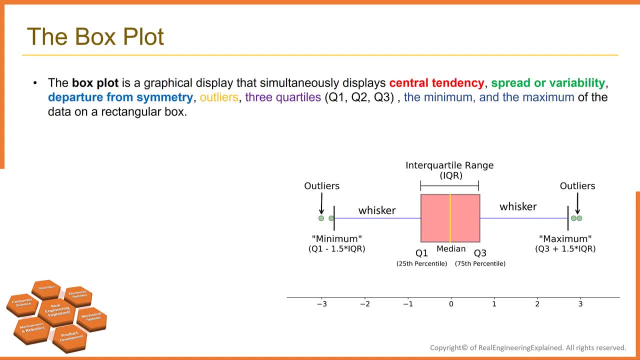 A box plot also displays the three quartiles of data, the minimum and the maximum of data on the rectangular box, which could be aligned either horizontally or vertically. This box encloses interquartile range with the left or lower line at the first quartile, Q1. 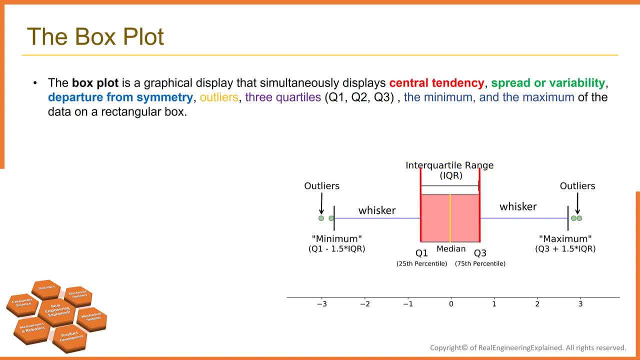 and the right or upper line at the third quartile, Q3.. A line is drawn through the box at the second quartile. This is the 50th percentile or the sample median. There are two lines at both ends which extend to extreme values. 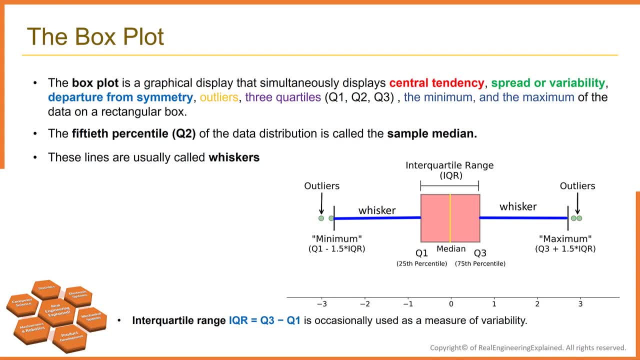 These lines are usually called whiskers. Some authors refer to box plot as a box and whisker plot. In some computer programs the whiskers only extend a distance of one and a half, multiplied to Q3 minus Q1, from the ends of the box. 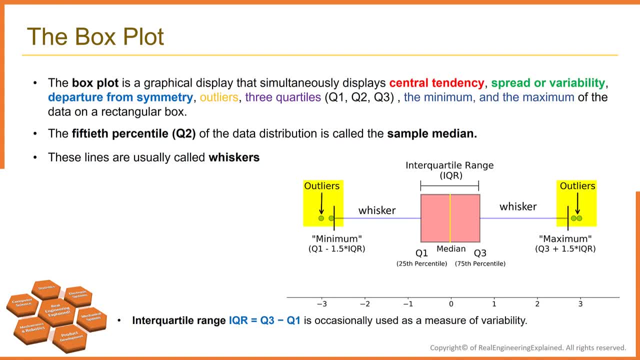 An observation beyond those limits are flagged as potential outliers. So always remember, use box plot to assess and compare the shape, central tendency and variability of sample distribution And look for outliers. Box plot works best when the sample size is at least 2.. 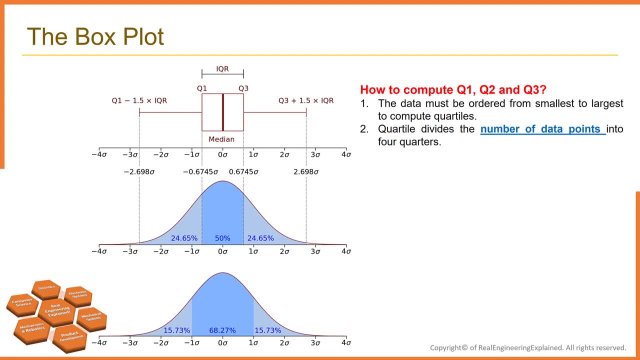 So the question is how to compute Q1, Q2 and Q3.. First, the data must be ordered from smallest to largest. to compute quartiles, Quartiles divides the number of data points into four quarters. The Q1, which is called first quartile. 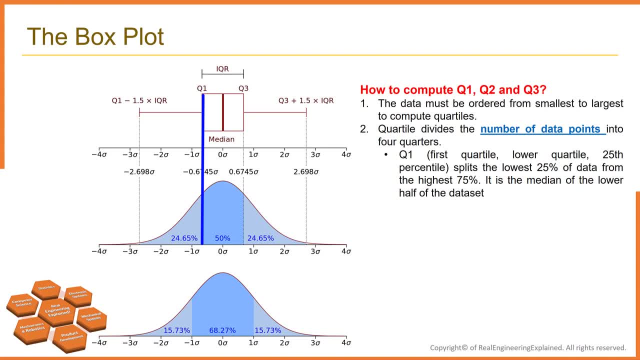 lower quartile- 25th percentile- splits the lower 25% of data from the highest 75%. It is the median of lower half of the data set Q2, or so-called second quartile median, or 50th percentile. 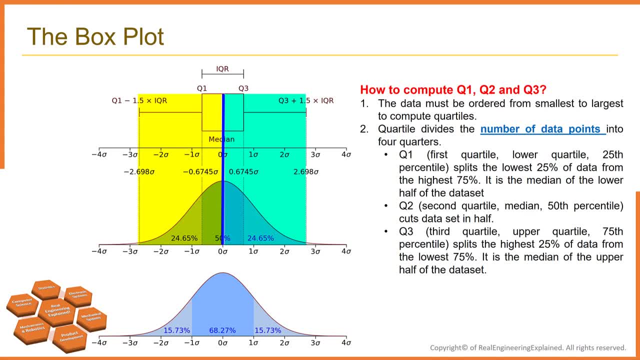 cuts data set in half. Q3, or so-called third quartile, upper quartile- 75th percentile splits the highest 25th of data from the lowest 75%. It is the median of upper half of data set. So, as you can see, 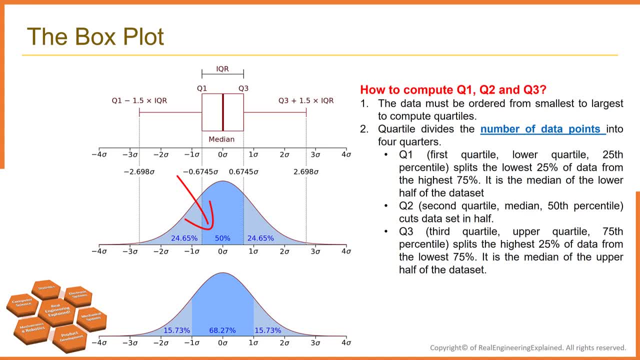 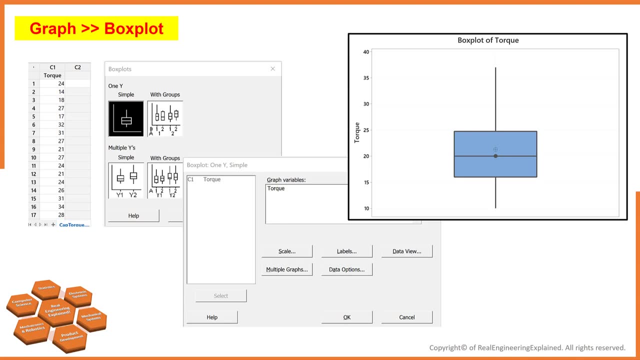 50% of data are between Q1 and Q3.. Just remember that this is the number of data between Q1 and Q3. Or interquartile range In Minitab. go to Graph, select Boxplot and then Simple. 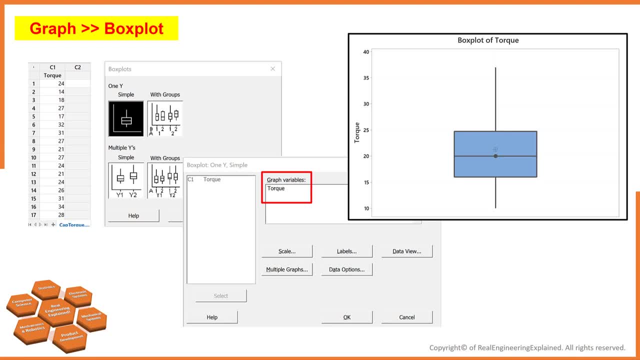 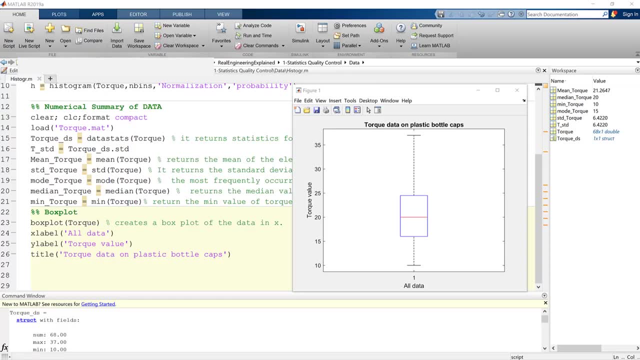 from Graph Variable, select Torque and hit OK. Here is the boxplot in Minitab. In MATLAB we can use Boxplot function to draw the boxplots. Run this part and here is the boxplot OK. 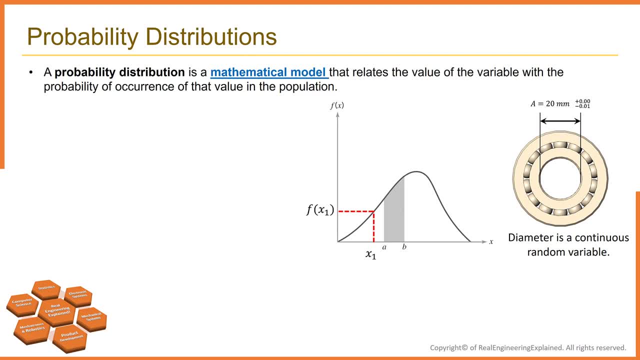 the fourth topic which I would like to talk about is probability distribution. The sample is a collection of measurements or observations selected from some larger population. For example, assume some measurements are obtained from a sample of ball bearings selected from manufacturing process. The population in this example. 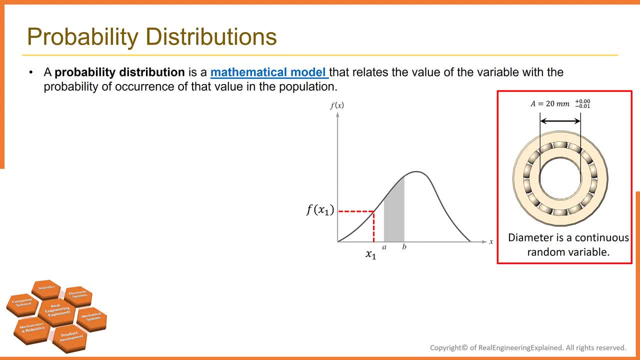 is the collection of all diameters produced by this process. A probability distribution is a mathematical model that relates the value of the variable, here the diameter on x-axis, with the probability of occurrence of that value in the population. We can visualize diameter as a random variable. 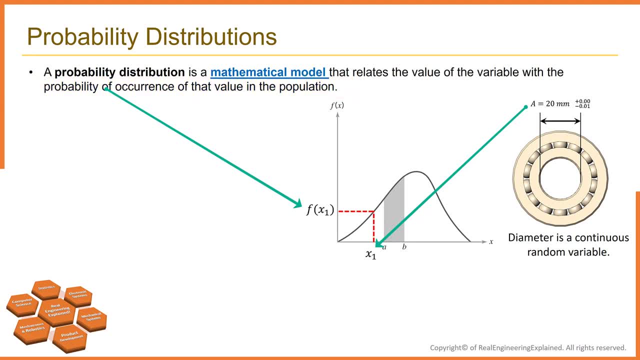 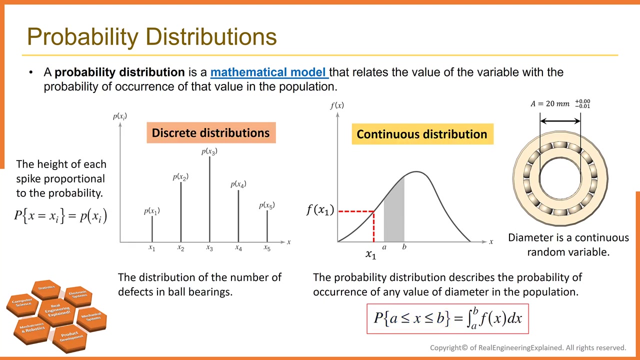 because it takes on different values. any number bigger than zero, Right? So remember this. the probability distribution describes the probability of occurrence of any value of diameter in the population, For example diameter between A and B in the whole population. There are two types of probability distributions. 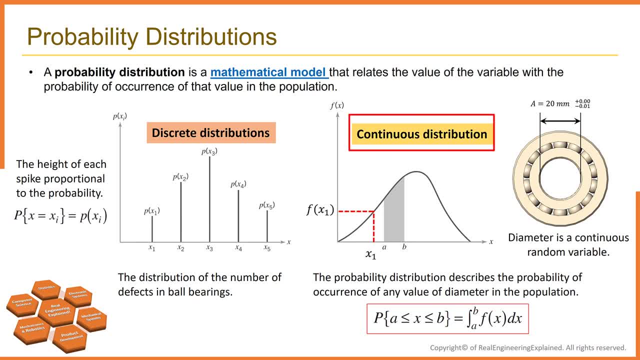 continuous distributions and discrete distributions. When the variable being measured is 0,. the variable being measured is expressed on a continuous scale like height or weight. it could take on any number. Its probability distribution is called a continuous distribution. In this case, the probability distribution of ball bearing diameter is continuous. 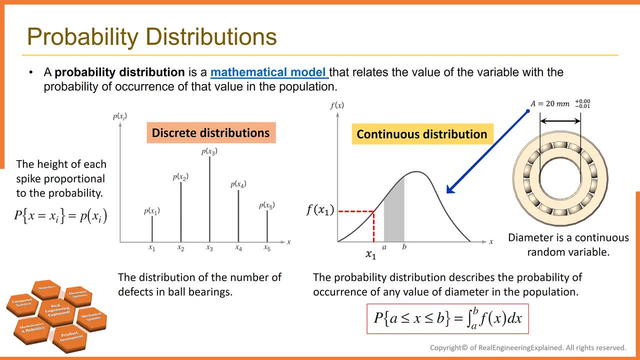 because it could take any number, For example 20.12 mm. There is another probability distribution, which is called discrete distribution, When the parameter being measured can only take on certain values, such as the integer 0,, 1,, 2, and so on. 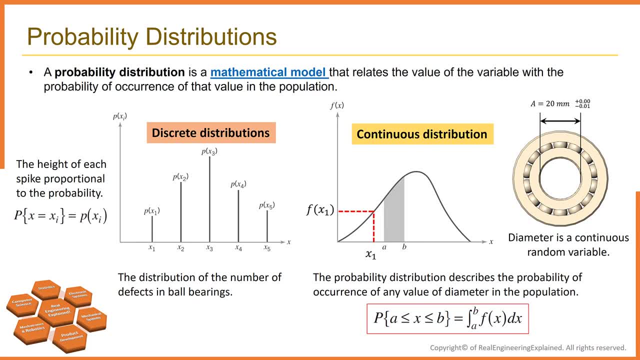 the probability distribution is called a discrete distribution. For example, the distribution of the number of defects in each ball bearing manufacturing line or the number of defects per day would be a discrete distribution. One day it could be 5,, another day 6,. 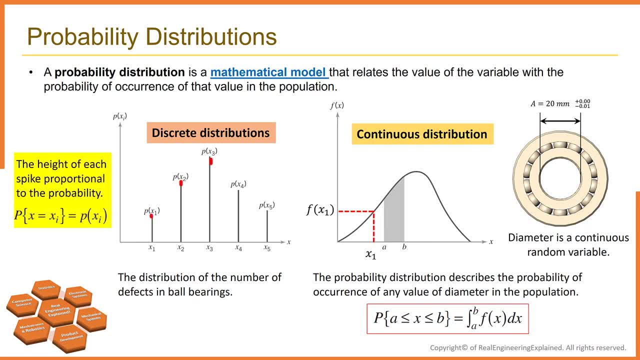 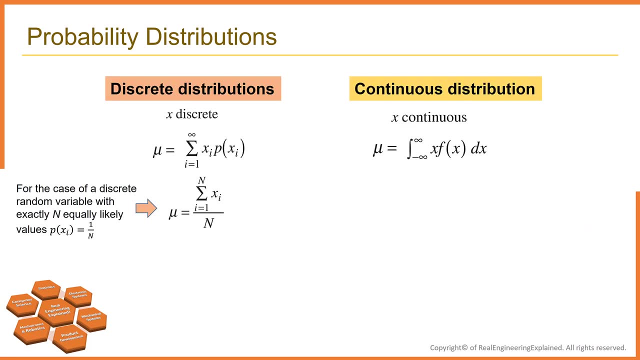 or another day- 0.. The height of each spike is proportional to the probability, The probability that the random variable x takes on the specific value xi as p. The mean mu of a probability distribution is a measure of the central tendency in the distribution or its location. 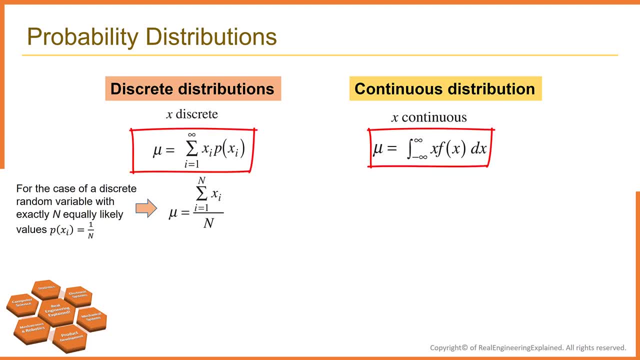 The mean is defined by this equation. For the case of a discrete random variable with exactly and equally likely values, the mean value can be computed with this equation. As you can see, the mean is simply the center of the mass of probability distribution. 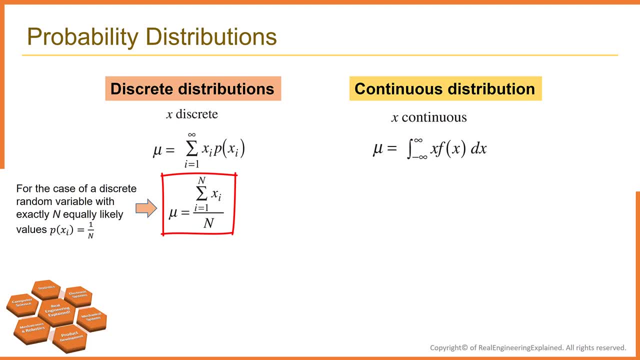 That's the summation of the all observations divided by the number of observations. Please note that the mean is not necessarily the 50th percentile of the distribution. Mean is not necessarily equal to the median. The scatter spread or variability in a distribution is expressed by the variance. 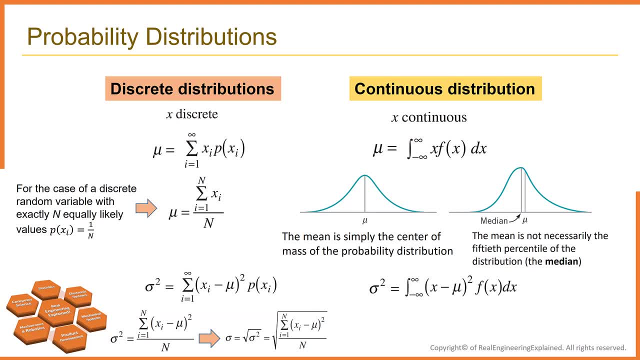 The definition of variance for discrete random variable with any equally likely values is the average square distance of each member of the population from the mean. The variance is expressed in the square of the units of the original value. The standard deviation can be defined as the square root of variance. 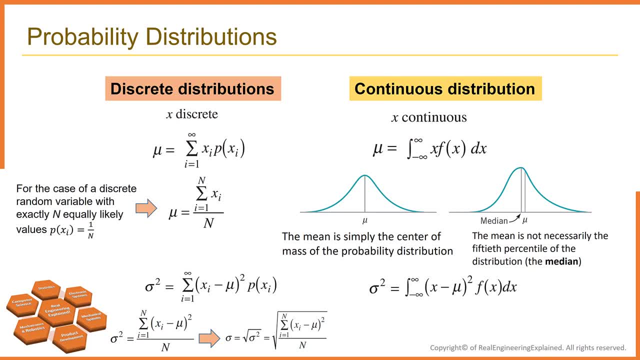 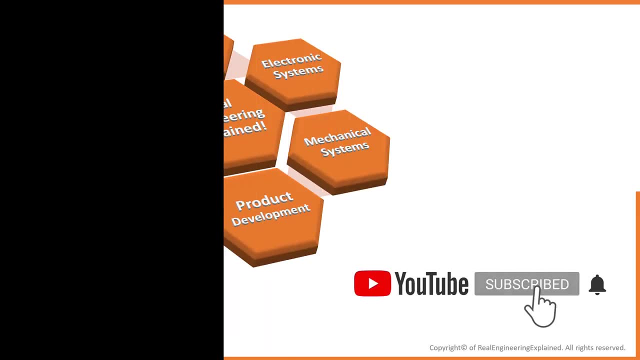 Alright, in this video we covered four basic terms in statistics: histogram, numerical summary of data, boxplot and probability distribution. We will discuss more about continuous and discrete distributions in this video series. We are going to release video series on different topics. 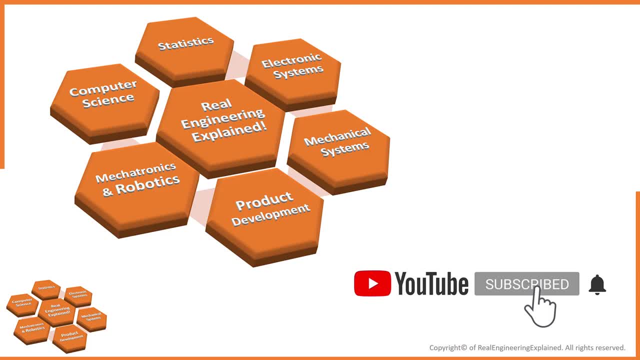 including application of statistics in manufacturing and quality control, robotics and mechatronics, industrial machine vision, system dynamics, finite element analysis, analysis with abacus, GD&T and Collins analysis, and many other interesting topics. Don't forget to subscribe to this YouTube channel. 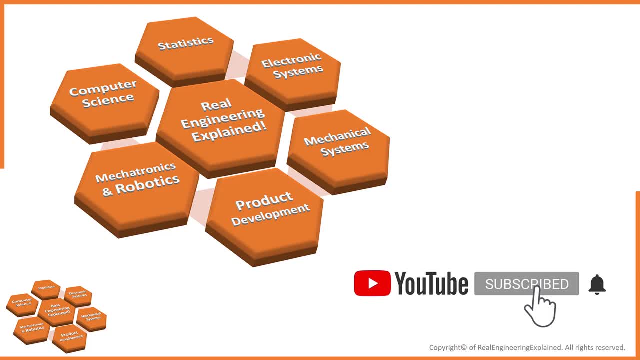 to get notified when a new video on this topic is released.